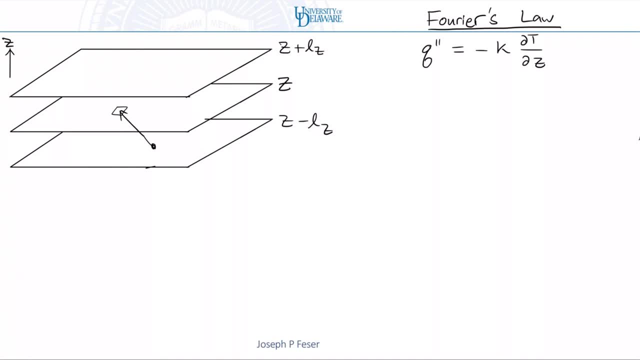 That is some position Z, that you know, all of the molecules in that plane are meant to have a particular temperature, And then all of the molecules in the plane above it are meant to have a- let's say, I don't know- a higher temperature. 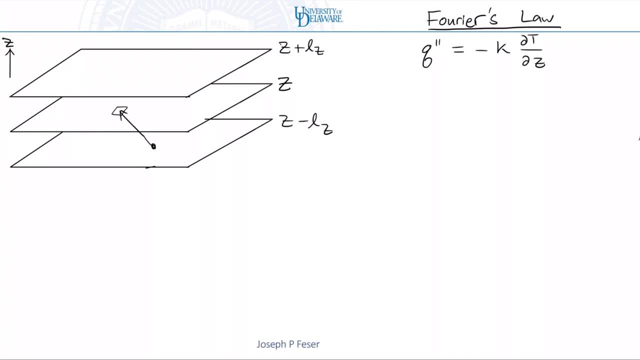 And the ones below it are meant to have a lower temperature. And so the question is: what is the net heat flux Through a little element of area that I'm highlighting in plane Z? Okay, so what do I know? So I would like to. 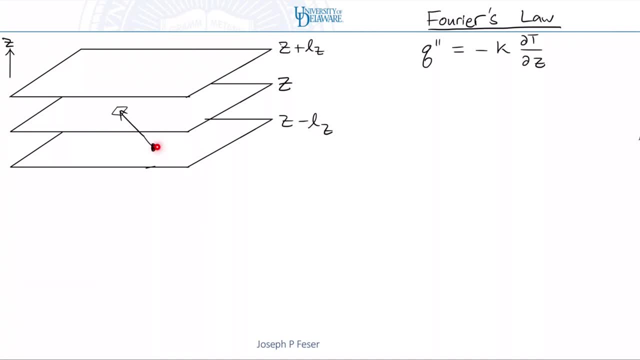 Okay, so I'm going to highlight a hypothetical molecule, or, you know, statistical set of molecules, coming from a position in the lower plane, And what I know is that, in order for this thing to have a different temperature, it has to be at least one mean free path away from. 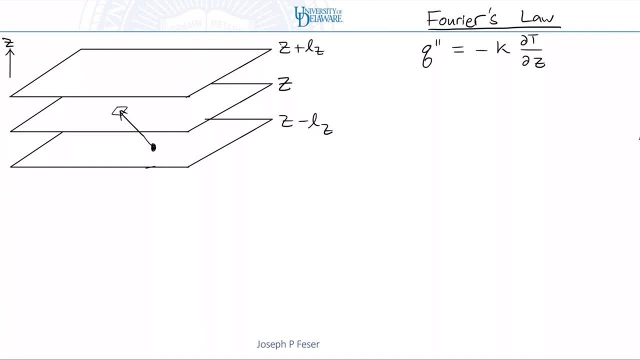 the patch that it's going to go through right, Because there has to have been a collision in order to establish a different velocity distribution of particles, which is essentially what defines the temperature. So what I'm going to do is I'm going to place these layers such that the particle arriving is a distance L away, where L is the mean free path. 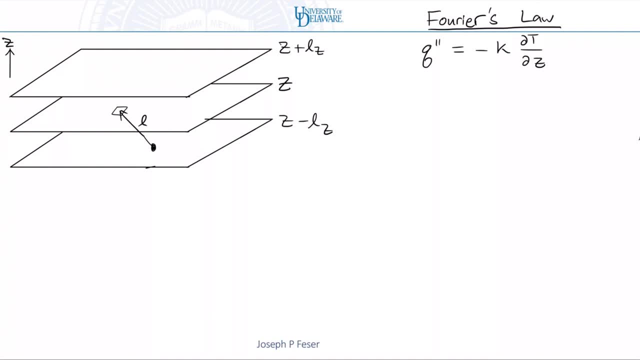 Because the particle doesn't necessarily have to be directly under the patch. it's not a perpendicular line at this point, It's just some vector connecting where the particle comes from to the patch that I'm interested in, And I can highlight an angle phi that defines the perpendicular portion of that. 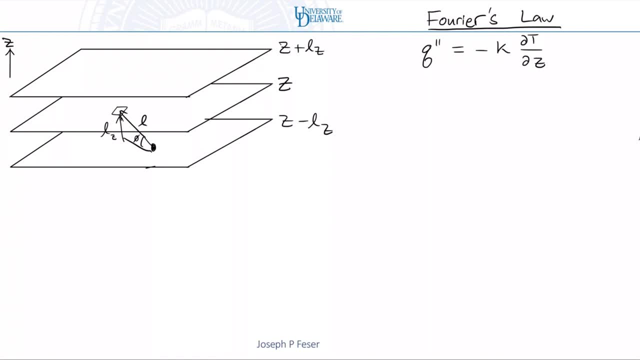 So if I take L sine phi, L cosine phi, or sorry, L sine phi, L sine phi, is that right? No hold on a second. let me redefine that. to make sure that I'm doing this consistently, Let me define this angle as phi, so that it's more like: 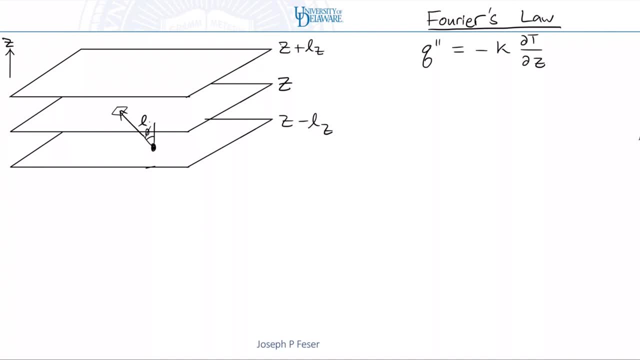 and this is meant to be like a perpendicular line now. So that basically defines a polar, a spherical polar angle between a perpendicular and everything else. So in other words, Lz is defined as L, times, cosine, phi, Okay, wonderful, Okay, so that defines the distance between planes. 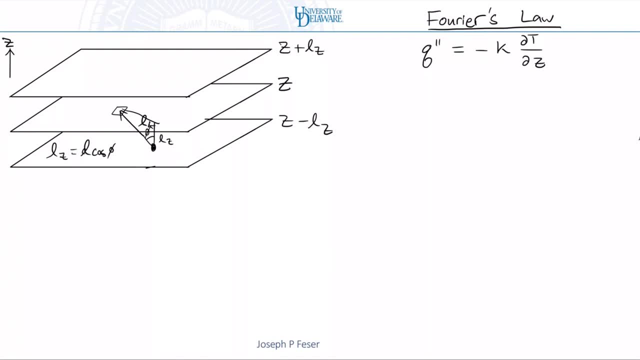 That's sort of the smallest distance I could possibly put the planes apart, And what I'll do is I will try to characterize the heat flux going through that little patch of planes. So I'm talking about this little patch right here. So what does that depend on? right? 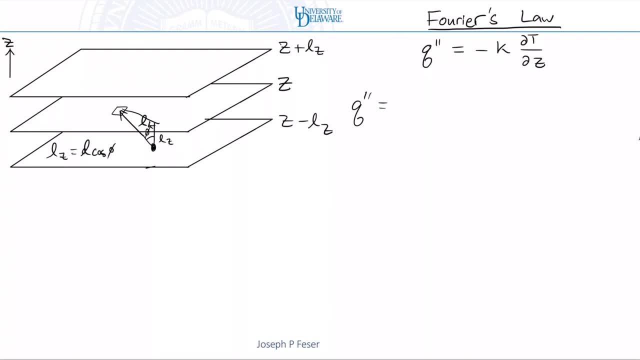 So it depends on: Well, what's the, What's the energy of that particle that'll be coming from that little highlighted point down here. So, what is the energy of that thing? I'm going to call that? I'll call the internal energy density U. 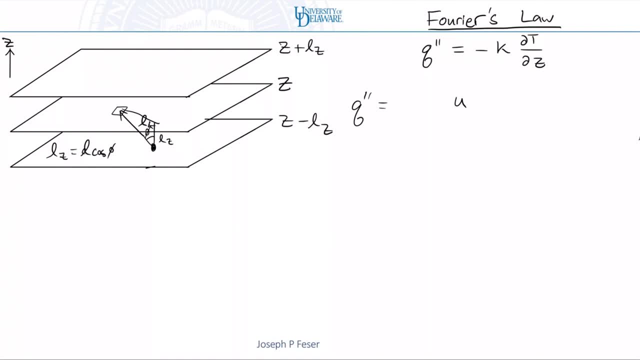 So it's going to travel up with speed- let's say vz- And so it's going to travel with energy. So I'm going to call that U evaluated at z minus Lz. so if I'm talking about this bottom energy carried by this bottom point, 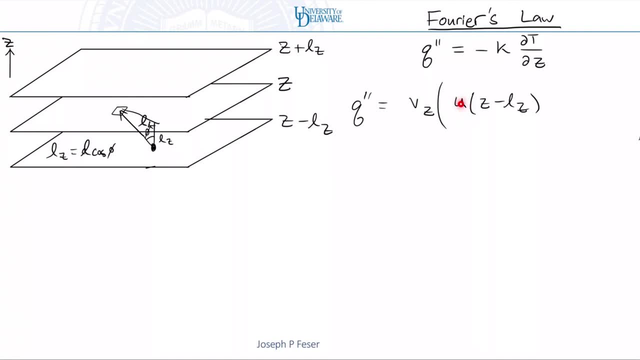 So this is meant to be the energy density, the internal energy density, And that I'm going to. What I mean by that is it's got energy density in a volumetric way. It's got energy density in a volumetric sense, so joules per meter cubed. 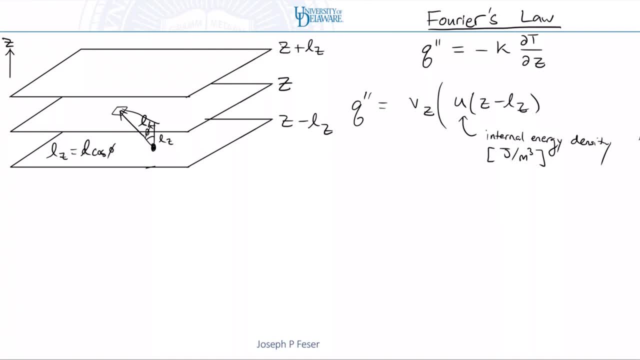 So this is the amount of energy density that is contained essentially by particles being emitted from plane z minus Lz. So that defines how much energy they have, And then this piece defines how rapidly they arrive. So And that vz is the projected velocity, right? 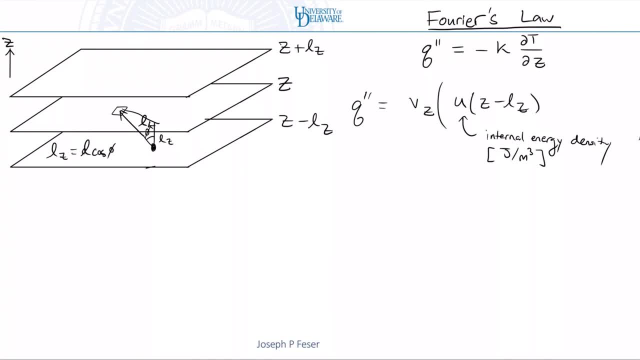 So that's the velocity in the z direction of typical particles arriving From that point. And of course, whatever the energy density is from this plane, only half of the energy density will end up going towards that interface. So I'll include a factor of half here. 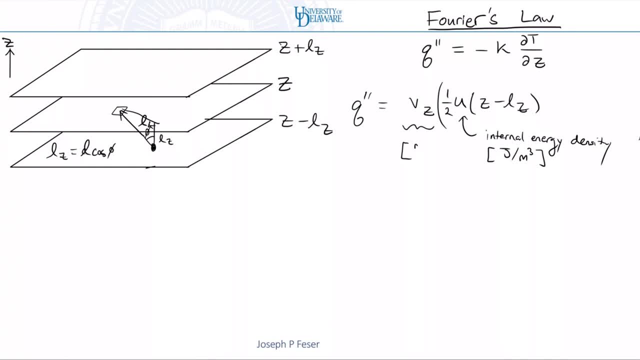 And let me check the units of this. So this is meters per second. So the energy arriving from the lower plane from this point is whatever the energy density was, So that's in joules Per meter, cubed Times the rate at which it gets there. 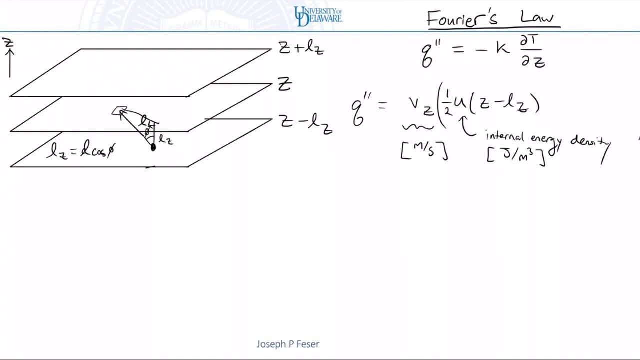 And if I check those units, it gives me joules per meter squared per second. That's the energy arriving from particles on the bottom. What about the energy arriving from up here? Well, that would create a negative heat flux, because that energy, if it's arriving from the top, then the energy would be going in the wrong direction. 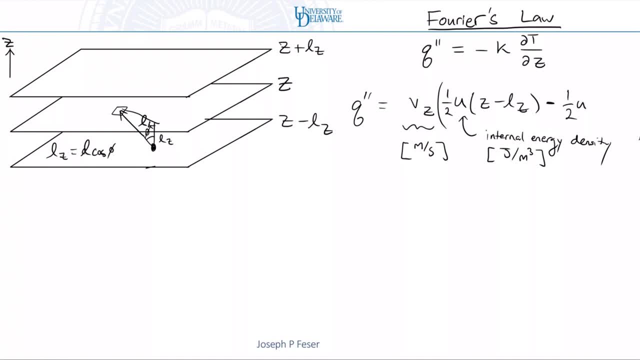 So I have to subtract a factor of half times U, Z plus LZ, And that gives me the energy you know coming through in the other direction, from the top side. Okay, So if I look at- oops, I did not mean to be highlighting. 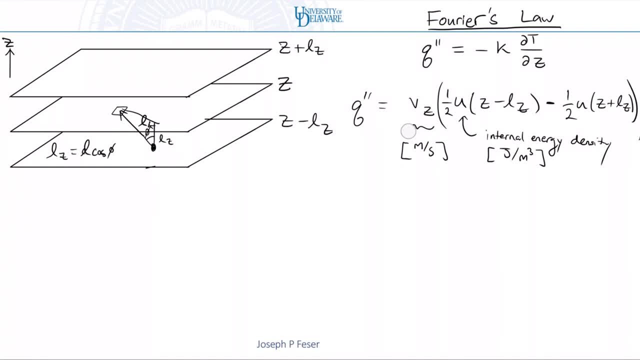 How did I do that? So let me erase this so I have some room to write here. So, and of course, the energy density. So this energy density, the internal energy density, is absolutely, Absolutely related to the temperature, right? 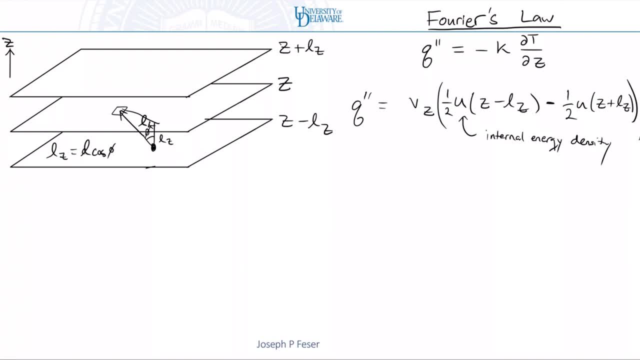 So in fact we- I think we- showed that the energy of a, the. yeah, at one point during the statistical thermodynamics chapter we should have shown that the energy density, or this thing U, at least for a monatomic gas, was three halves KBT. 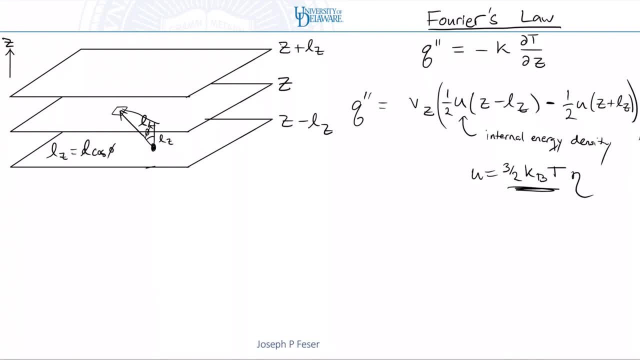 That's the energy. That's the energy per molecule times the number density of molecules. So specifically, this is what I mean about the internal energy density. All right, So we'll come back to that in a second. Okay, So now, if I look at what this thing is now, the energy density actually depends on, you know, the temperature. 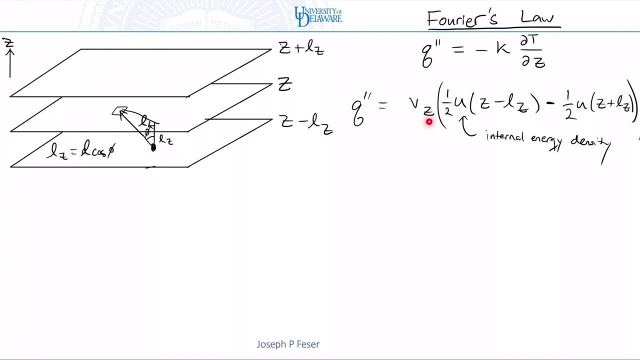 But also the this speed, the average speed of something coming up will depend on the temperature And the mean free path depends- well, LZ depends on where the particle came from. So I can kind of see that this isn't exactly rigorously correct yet. 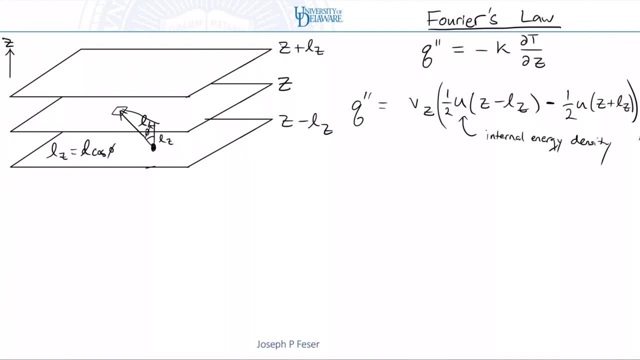 What we need to really do is take a directional average. So, depending on where this particle came from, it might have a different, you know- it might have a different VZ, it might have a different velocity and it might have a or VZ anyway, and it might have a different LZ. 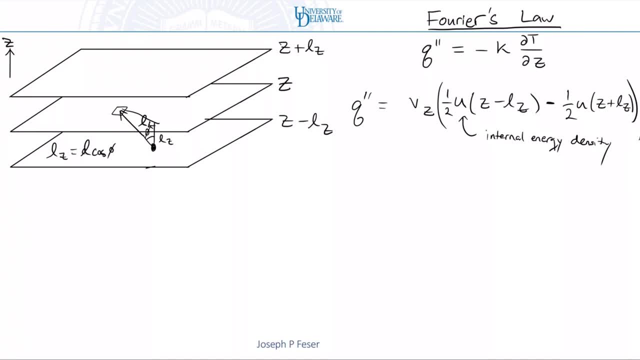 And so we'll have to do a directional average at some point. But let me, just before I do that, let me do a one other thing, which is I'm looking at, looking at this, and I see that I have something that looks like, you know, a function evaluated at L minus LZ and another function evaluated at Z minus LZ. 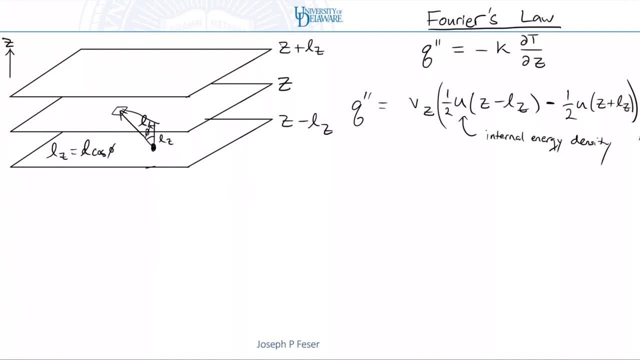 And I mean it seems to me that what we should do here is think about doing a Taylor expansion right. I'm interested in relating the heat flux To what's going on at a point in the central plane. That's really what Fourier's law relates to. 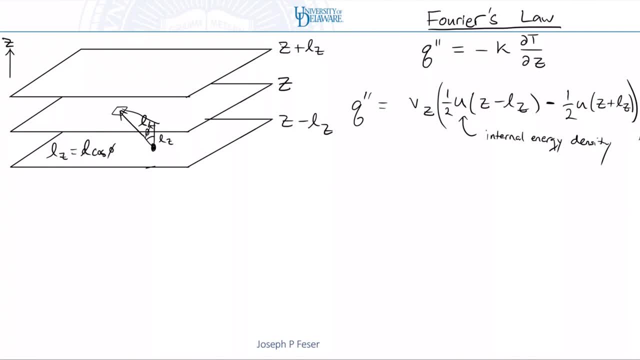 And I have terms that look like: you know a number, you know minus a small number and a number plus a small number. That's like sort of begging us to do a Taylor expansion. So let's do that. So if we do a little Taylor expansion in here, 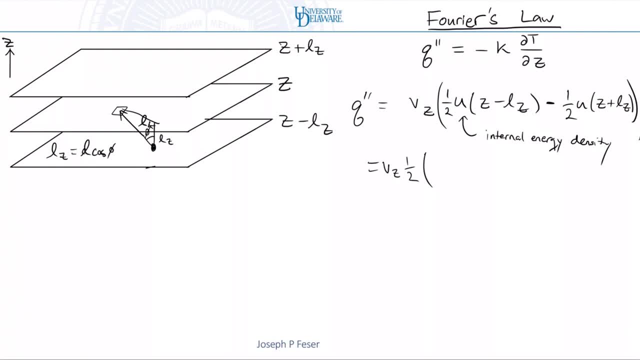 The first term. So this term Expands to give us U evaluated at Z minus LZ D U D Z, evaluated at Z minus U, Z minus LZ D U D Z. So if I, if I take a look at it, Well, what I'll see is that I've got like two terms that cancel each other and two terms that are additive. 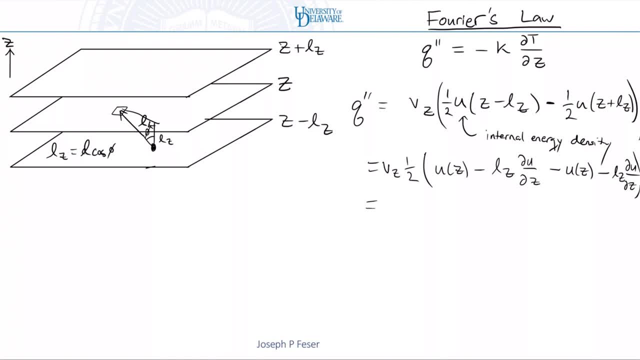 And so if I put it all together, I get: And, by the way, the two terms that are additive will cancel the factor of half, And so that'll give you a V Z L Z D U D Z. Well, that's looking a little bit like Fourier's law, but not quite. 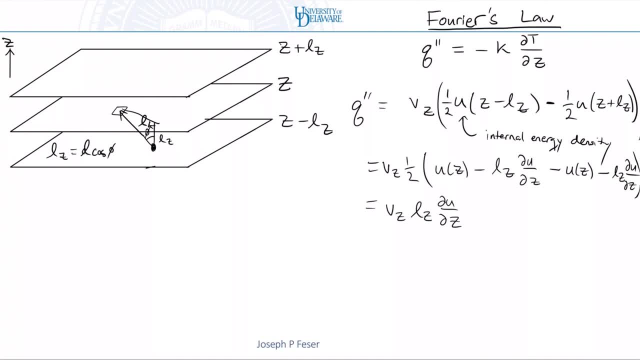 I was really interested in well a couple of things. So I've already- I've already- sort of indicated that we probably need to do a directional average over all The possible places that this particle could have come from. But the other thing is we need to relate the internal energy to temperature. 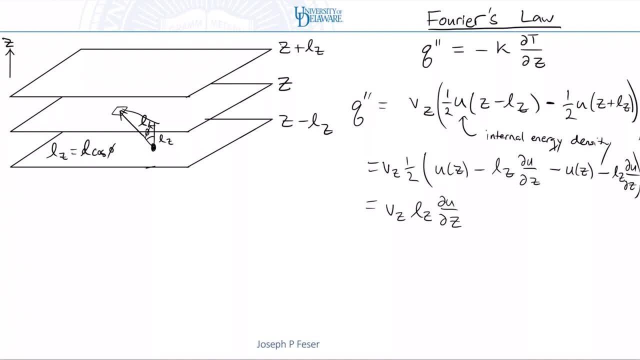 Let's do the first. Let's let's do the directional average first. That's easier. So V Z L Z, I can write as V times L times cosine squared phi, And then I can do the direction. So I need to do two averages. 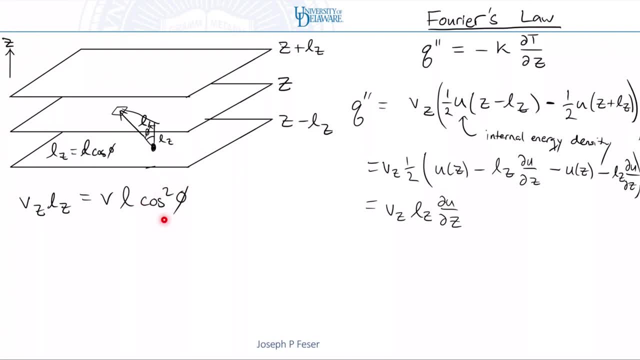 I need to do the average over the probability that this thing Came over from all possible different angles. But I also need to do a directional average over all the possible velocities that could have been coming up from the, from the bottom plane. So if I do those directional averages, 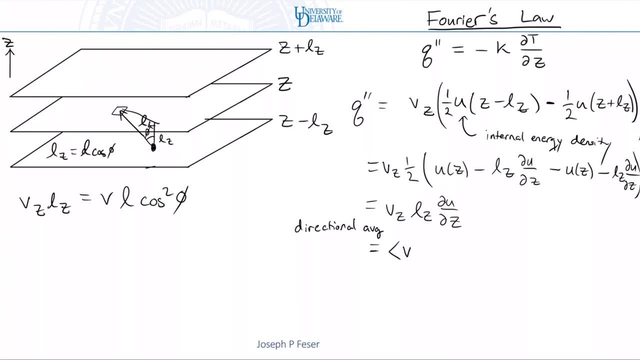 Um, I'll get an average velocity Average. um, well, I don't really have to average, the mean free path. It's already sort of pre averaged and um, then I need to to take. okay, so I'll keep. I'll just keep the D U D Z there. 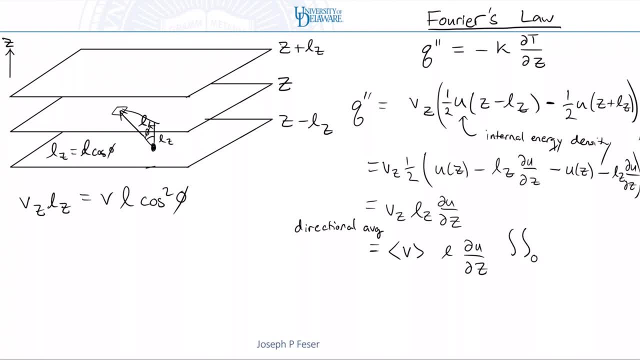 But then I need to do this directional average of um cosine squared, uh, in spherical coordinates, um, if I do that, what I'll what I'll get is that, um, this top piece is going to give you something that looks like two thirds times pi. 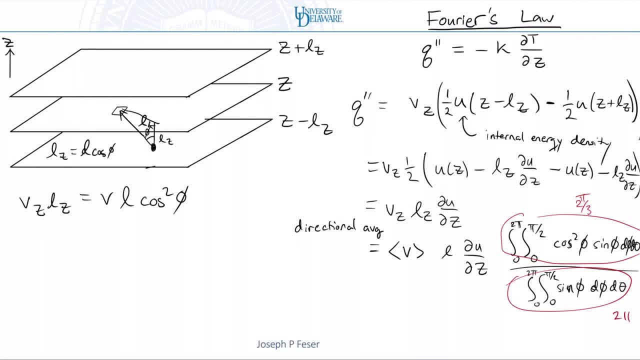 and the bottom piece will give you something that looks like two pi, And so the net result is that you get a factor of one third out of all that, And so the final answer, which I guess I'll write over here somewhere, is that, you know, this thing is one third times the average velocity, times L, the mean free path. 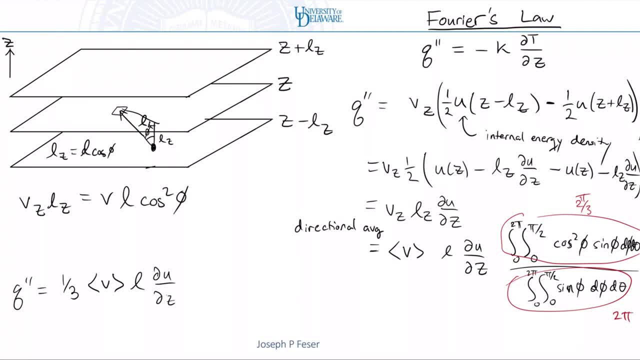 times du dz. Okay, How does? how does u depend on temperature? I need to think about this a little bit carefully because it says partial derivative here. It's really supposed to be in the z direction only And u depends on. is a state function essentially right? So like u or internal? 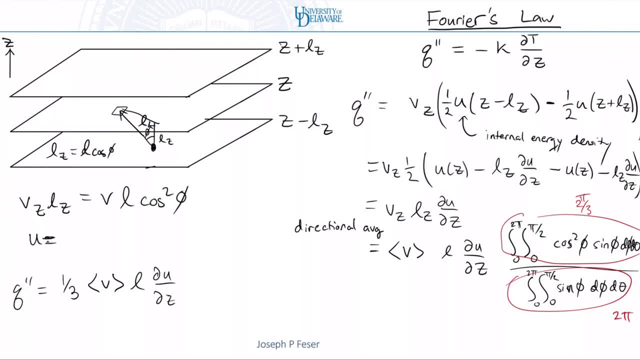 energy always sort of depends on, or it's a function of, the temperature, the volume and the number of particles. right, But you know, if I'm trying to, if I'm only considering the fact that temperature can change between layers, and you know my state function looks like this. then what I mean by you know, taking the 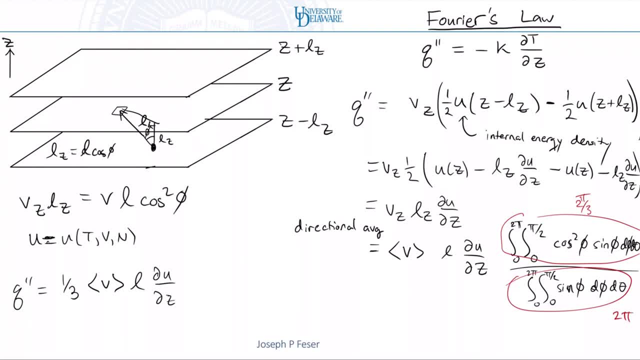 derivative with respect to temperature is to take the partial derivative at fixed volume and number of particles, In which case what you'll see is that, basically, this thing is one third times du dt at constant Constant volume and number of particles times VL, times dt dz, And this thing is nothing but the heat. 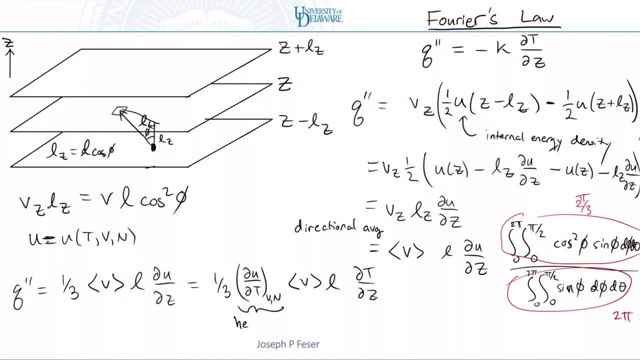 capacity, or especially because- so note that I had written the internal energy density up up here volumetrically, So this was supposed to be in joules per meter cubed, And that means that when I come down here and I need to do this derivative, what I really mean is that this is the volumetric heat. 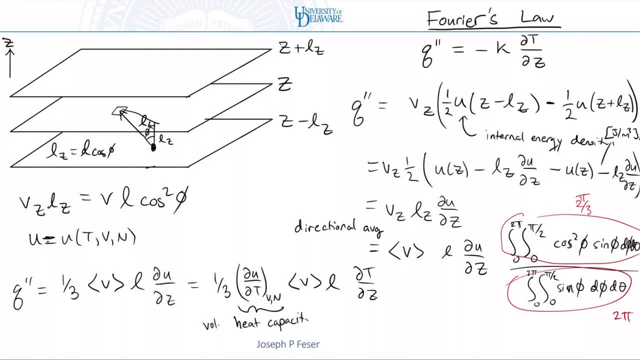 capacity at constant volume. So, in other words, this thing is CV And it's written on a volumetric basis. And one thing that I was a little bit lazy about was the minus sign, So you'll notice that up here there was a minus. 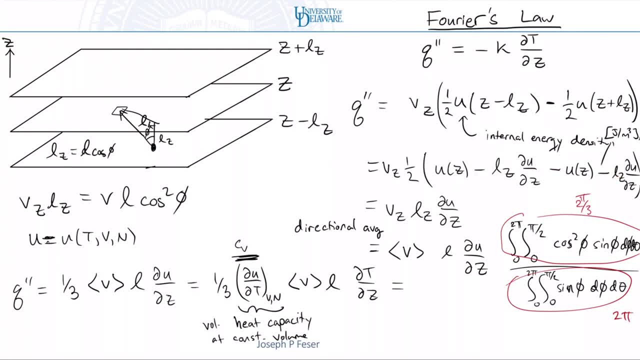 sign that came along with the LZs that I forgot to carry along, So let me just patch that in here, here, here, here. And so now what I have, if I just compare these two things: Oops, not that one. 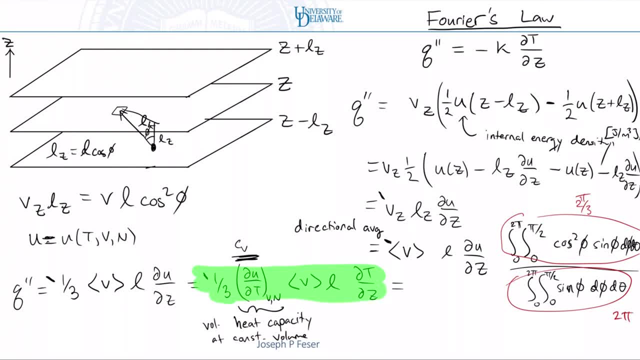 So let's compare this to this And voila, We see that, basically, you know, by doing a basic accounting of the heat flux, what we have is something that relates the heat flux to the local temperature gradient And there's a constant. 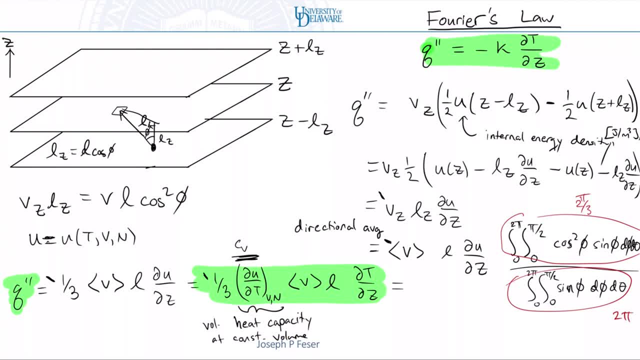 of proportionality that sits in between, And so we can identify what that is right. So that thing must be the thermal conductivity, And the value of the thermal conductivity is apparently that the thermal conductivity is one-third CVL, where L is the mean. 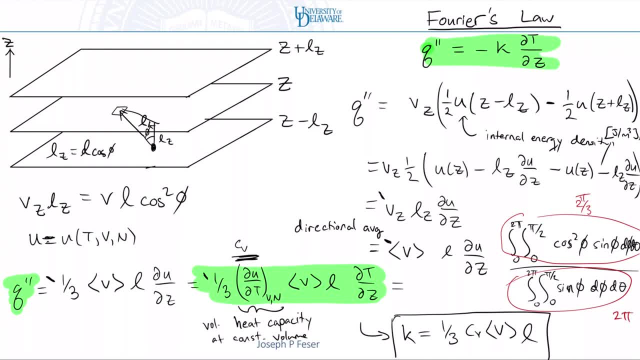 free path, And so that's really pretty much all there is to it, So you can do this. So we've identified that the thermal conductivity is one-third CVL from our, you know, from what we know about the Maxwell distribution for velocity. 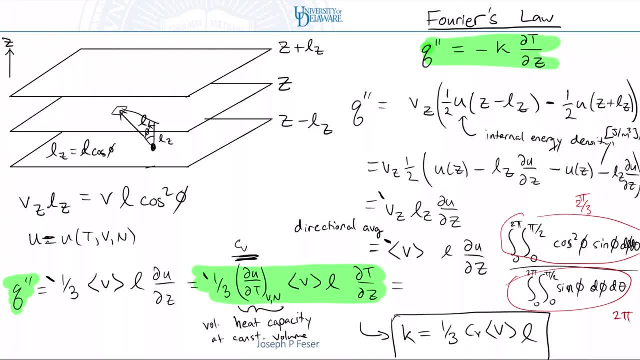 And as soon as you do, this addresses- And so, even if each hacks does that- various velocities. we can figure out what the average velocity is in terms of the mass and the temperature. We can figure out the mean free path in terms of the number, density of gases and the size of the particles. We can figure out the heat capacity in. 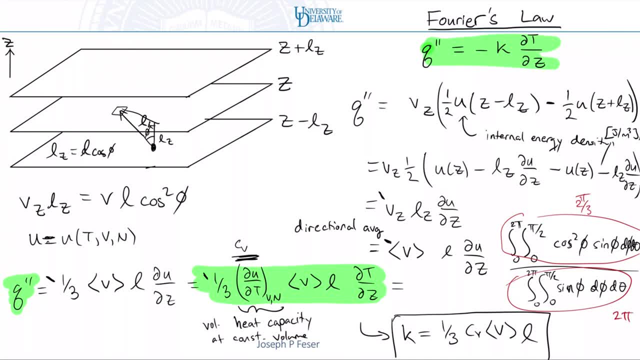 terms of. let's see, what does he capacity depend on? that only depends on the number, density of particles, basically. And so for a monatomic gas, and so we can figure out what CVL are from all those coefficientoptions, and L are from all of the previous things that we've learned and I'll do. 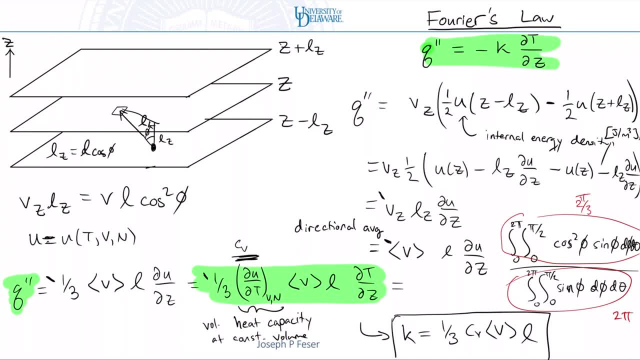 that in the next slide and calculate the thermal conductivity based on microscopic principles. so how awesome is that that's? there's a lot of. so you can do this for pretty much like this kind of technique for every type of transport property. I'll show you how to do it for viscosity and for molecular diffusivity. 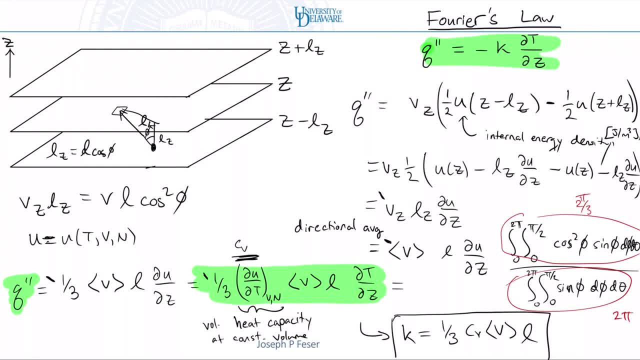 but the bottom line is that, like you can, you can follow this kind of approach to get almost any microscopic property. later I'll show you an even better way to do this. so there are. there are some small. it's hard, to hard to talk about yet, but there are some small discrepancies in the way that we did.